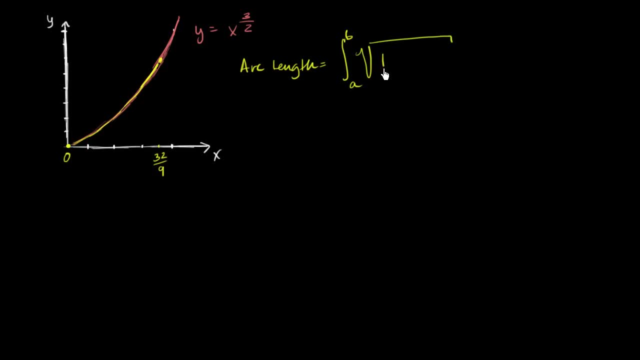 and then how we apply it. So it's the square root of one plus f, prime of x squared dx, And in this case that's going to be, it's going to be the definite integral from zero to 32 over nine of, I should say, the square root of one plus. 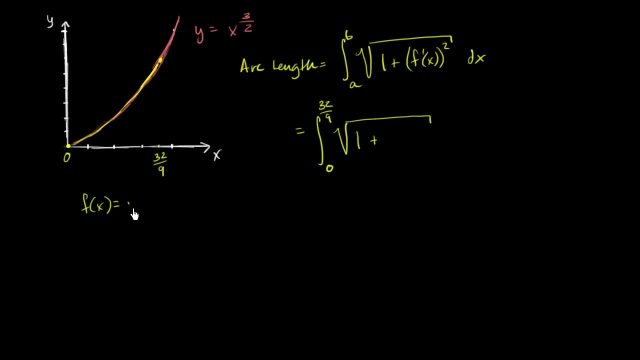 now what's the derivative? If f of x is x to the three halves, then f prime of x is going to be three halves x to the one half. And we picked this particular function because it simplifies quite well when we put it under the radical. 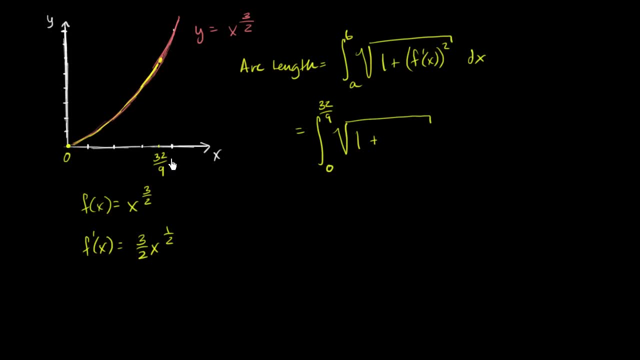 It's fairly straightforward to find the antiderivative, So we've done a lot of engineering of this problem to make the numbers work out, But let's just go through it. So this is f prime of x. F prime of x squared is going to be this quantity squared. 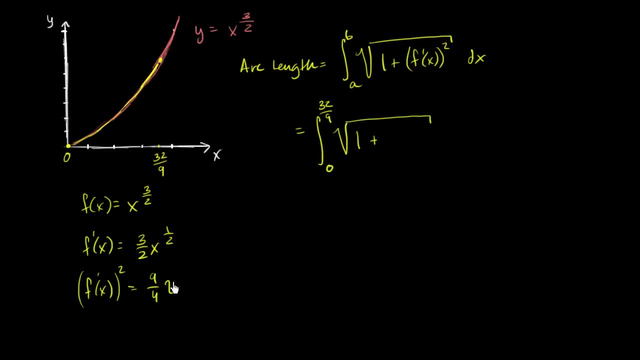 It's going to be nine over four x to the one. half squared is x, So one plus nine fourths x, dx. And so now we just have a definite integral that we know how to solve this type of thing, And you might be able to even do this in your head. 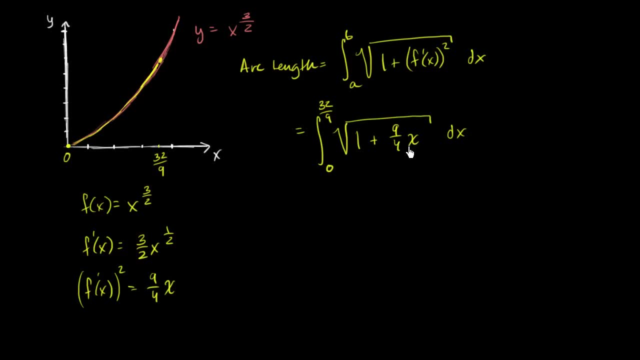 essentially do the u-substitution, Say: okay, I have one plus nine fourths x, It's derivative is nine fourths. I can kind of engineer that if I want, But instead I'm just going to do straight up u-substitution. 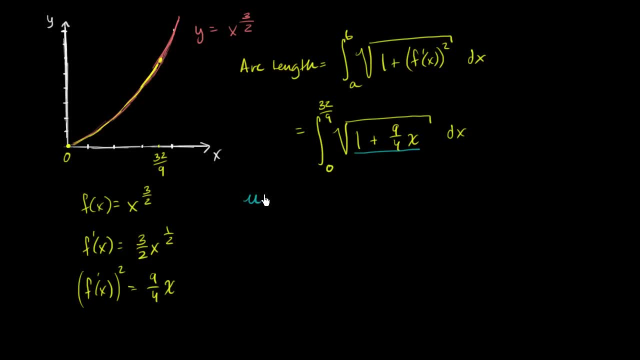 So u-substitution. So if I say u is equal to one plus nine over four x, Then we know, let's see, du dx would be: du dx is going to be equal to nine fourths. Or we could say: du is equal to nine fourths dx. 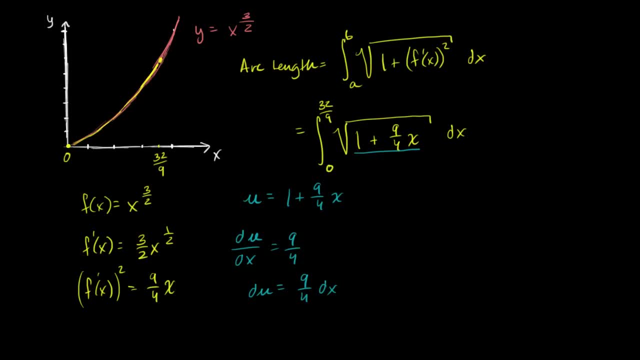 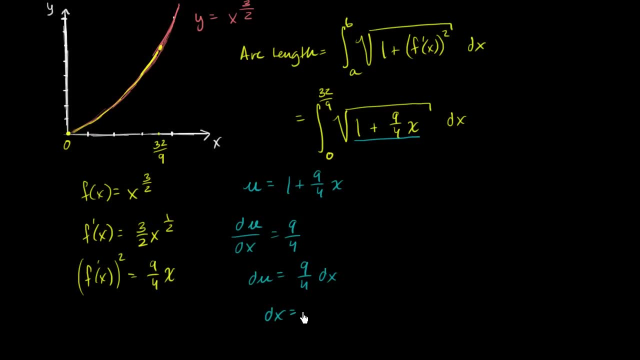 Or we could say dx. or we could say- let me scroll down a little bit- We could say dx is equal to- I'm just going to multiply both sides times four ninths: It's equal to four ninths du. And then we just have to change the bounds of integration. 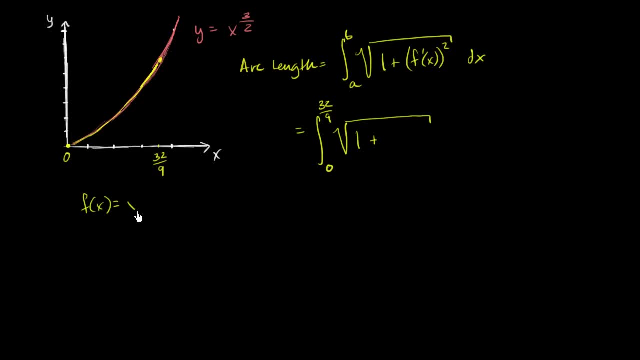 now what's the derivative? If f of x is x to the three halves, then f prime of x is going to be three halves x to the one half. And we picked this particular function because it simplifies quite well when we put it under the radical. 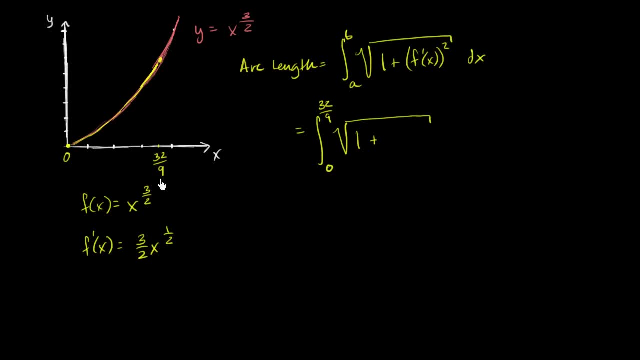 It's fairly straightforward to find the antiderivative, So we've done a lot of engineering of this problem. the numbers work out well, but let's just go through it. So this is f prime of x. f prime of x squared is going to be this quantity squared. 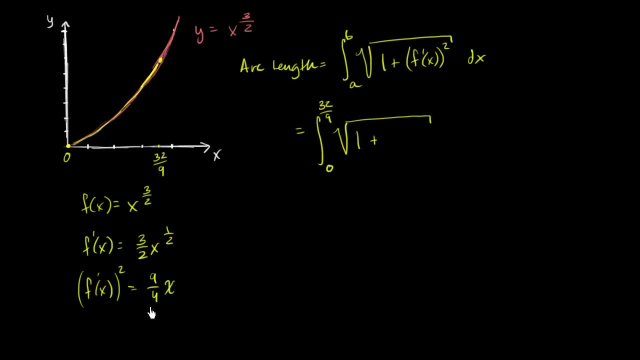 it's going to be nine over four x to the one. half squared is x, So one plus nine fourths x, dx. And so now we just have a definite integral that we know how to solve this type of thing, And you might be able to even do this in your head. 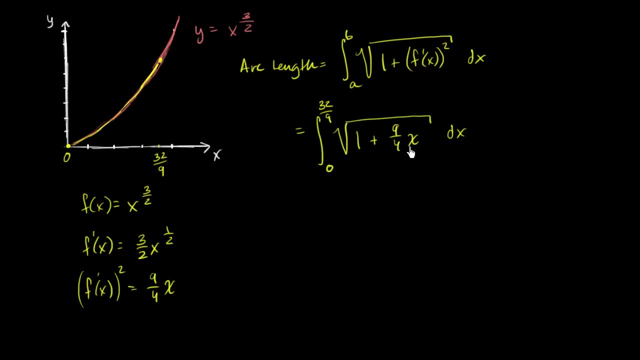 essentially do the u substitution say: okay, I have one plus nine fourths x, this derivative is nine fourths. I can kind of engineer that if I want, but instead I'm just going to do straight up: u substitution, So u substitution. so if I say u, 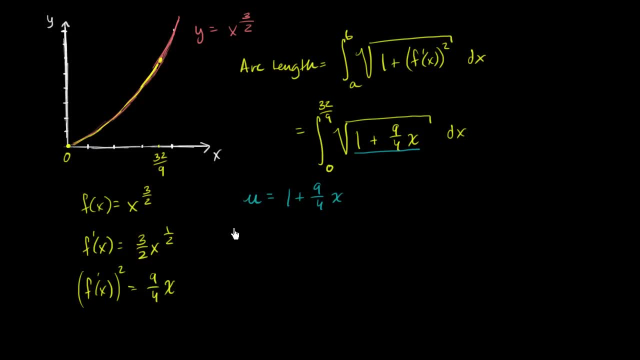 is equal to one plus nine over four x, then we know, let's see, du dx would be: du dx is going to be equal to nine fourths. or we could say du is equal to nine fourths dx. or we could say dx. 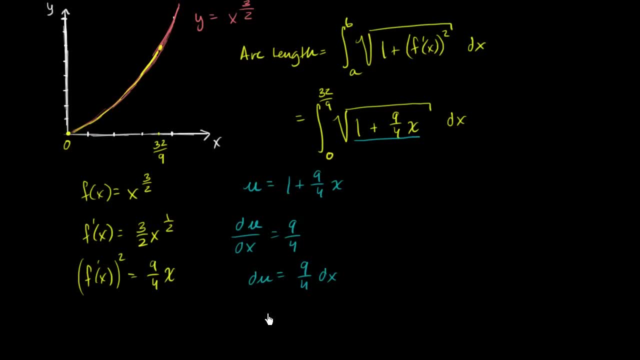 or we could say- let me scroll down a little bit- we could say: dx is equal to- I'm just going to multiply both sides- times four ninths is equal to four ninths du, and then we just have to change the bounds of integration. 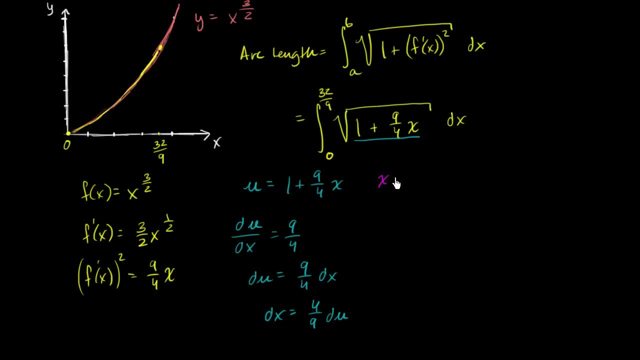 When x is equal to, when x is equal to zero, then u is going to be equal to nine. fourths times zero is zero, so u is going to be equal to one. and when x is equal to 32 over nine. 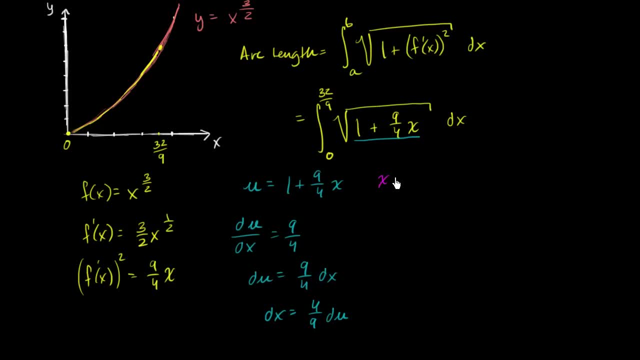 When x is equal to, when x is equal to zero, then u is going to be equal to nine. fourths times zero is zero, So u is going to be equal to one. And when x is equal to 32 over nine. 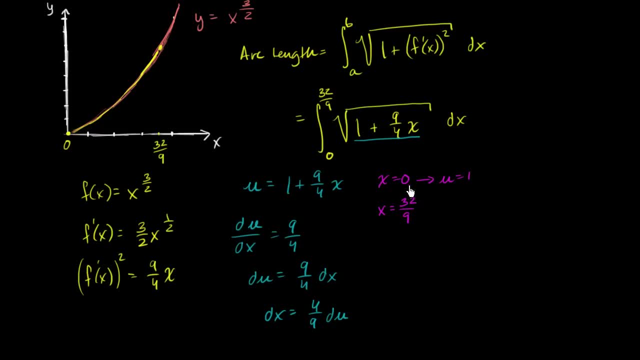 32 over nine and this is why that number was picked. what's u going to be equal to? 32 over nine times nine. fourths is going to be 32 over four, which is going to be eight plus one. So that worked out very nicely. 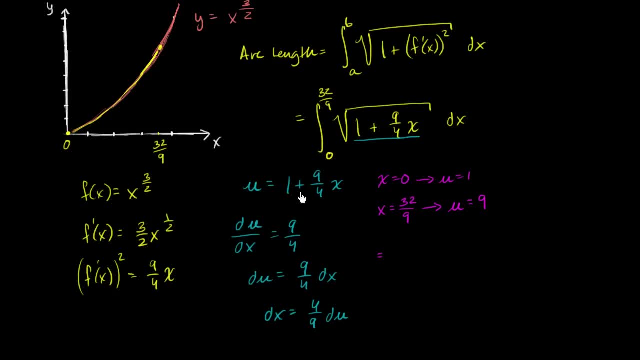 Imagine that. So there we have it. So this is going to be equal to. this is going to be equal to the definite integral. Actually, let me make it clear. This is what is equal to this: The definite integral from u is equal to u is equal to one. 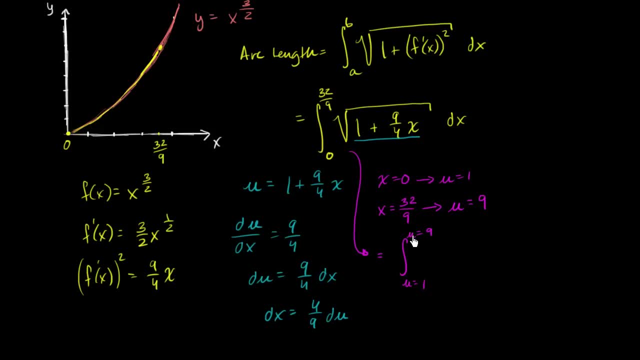 to u is equal to nine. I'm going to make it very explicit that I'm dealing with u now Of the square root of u instead of dx we have. dx is four ninths du. Let me do it this way: Square root- whoops. that's not the right color. 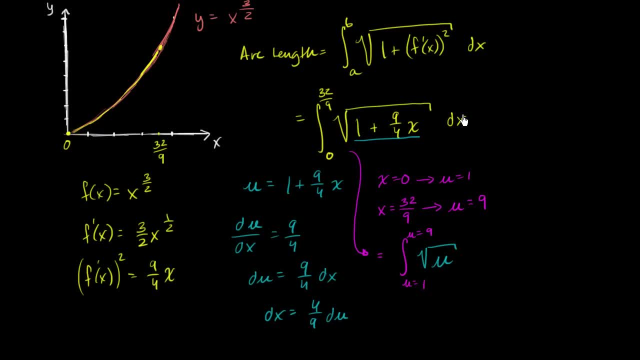 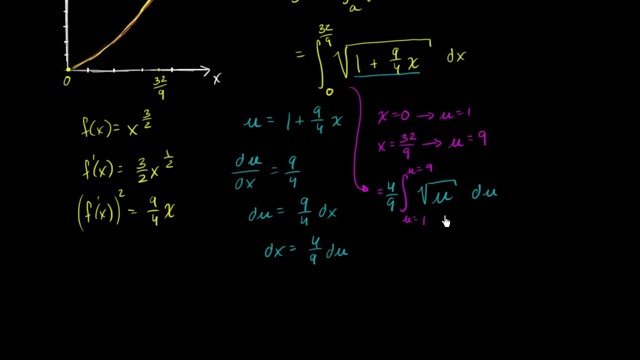 Square root of u instead of dx. we have times four ninths du And I'm just going to take the four ninths and stick it out here. Four ninths du And we know how to apply the fundamental or the second fundamental theorem of calculus here. 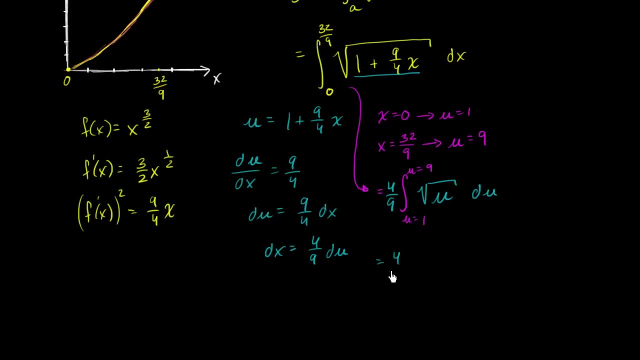 to evaluate this definite integral. This is going to be four ninths times. the antiderivative of the square root of u, which is the same thing as u to the one half, is going to be u to the three halves. And then we divide by three halves. 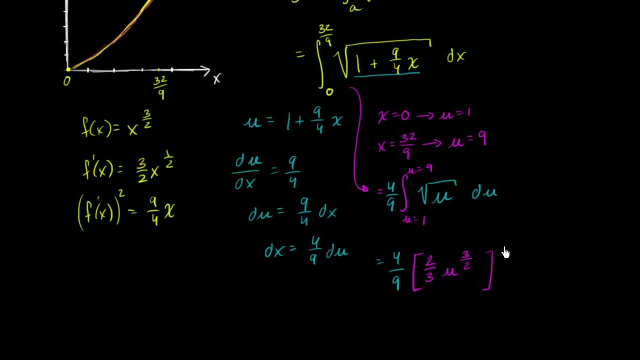 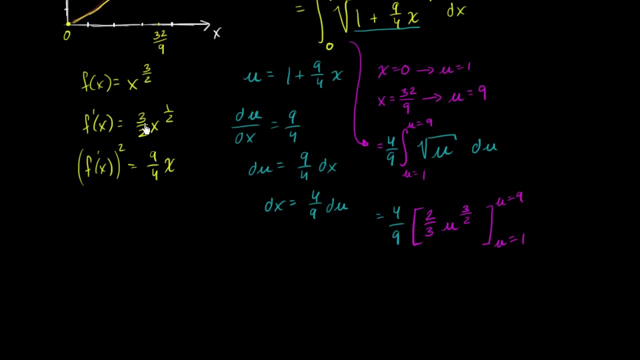 which is the same thing as multiplying by two thirds, And we're going to evaluate that at: u equals one, u equals nine and u is equal to one, And so we're in the home stretch here. This is going to be equal to four ninths. 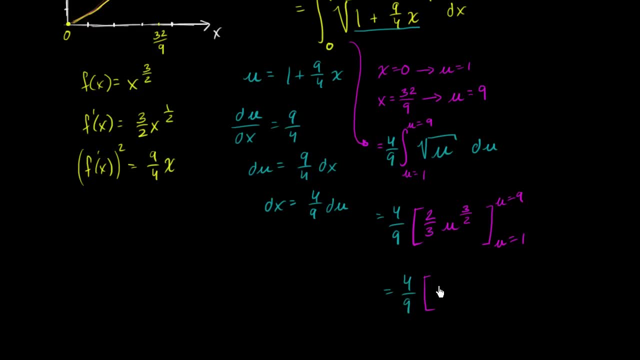 times, let's see two thirds times nine to the three halves, minus two thirds times one to the three half, So nine to the three halves, that is, let's see the square root of nine is three and the square root of nine is 27.. 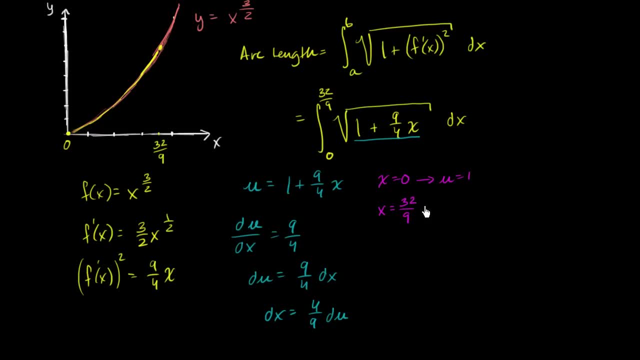 32 over nine, and this is why that number was picked. what's u going to be equal to? 32 over nine times nine. fourths is going to be 32 over four, which is going to be eight plus one. So that worked out very nicely. imagine that. 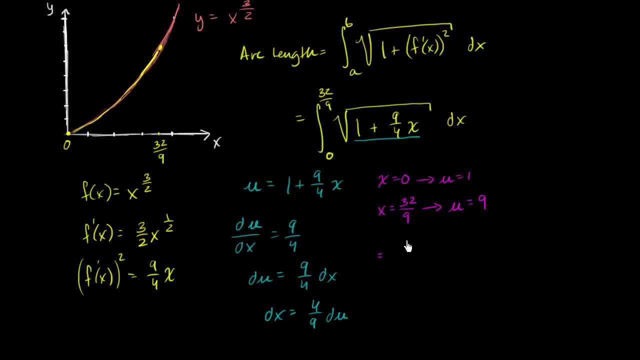 So there we have it. so this is going to be equal to. this is going to be equal to the definite integral. actually, let me make it clear. this is what is equal to this: the definite integral from u is equal to. u is equal to. 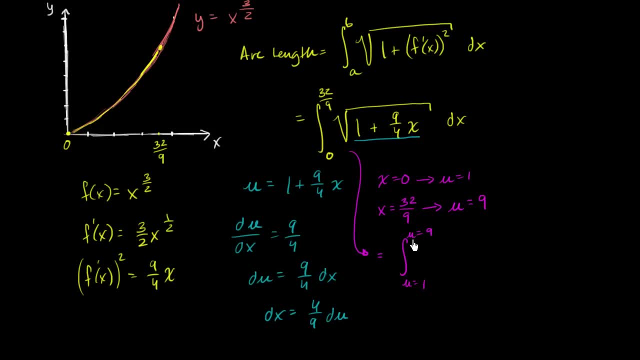 u is equal to one to u is equal to nine. I'm going to make it very explicit that I'm dealing with u now of the square root of u instead of dx we have. dx is four ninths du. Let me do it this way. 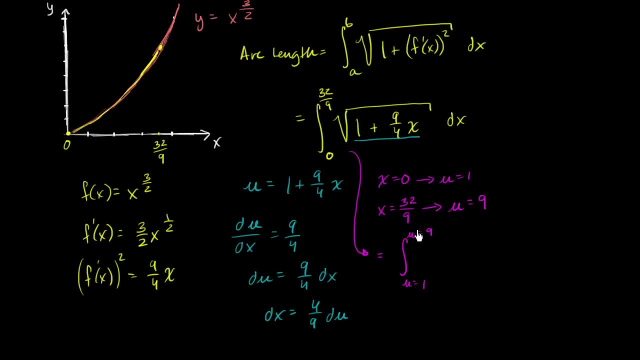 Square root- whoops, that's not the right color. square root of u instead of dx. we have times four ninths du, and I'm just going to take the four ninths and stick it out here. Four ninths du. 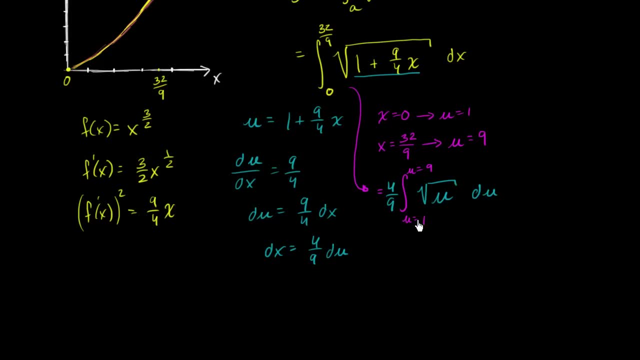 and we know how to apply the fundamental or the second fundamental theorem of calculus here to evaluate this definite integral. This is going to be four ninths times the antiderivative of u, of the square root of u, which is the same thing as u, to the one half. 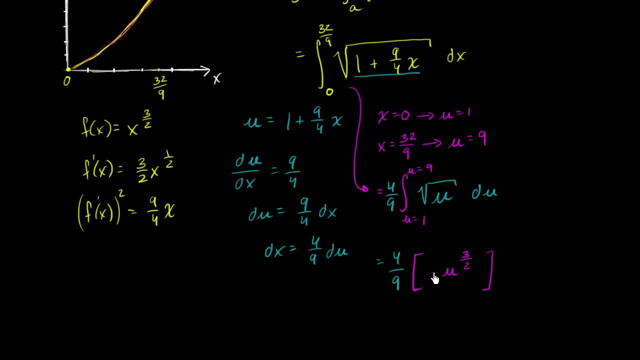 is going to be u to the three halves, and then we divide by three halves, which is the same thing as multiplying by two thirds. we're going to evaluate that at: u equals nine and u is equal to one, and so we're in the home stretch here. 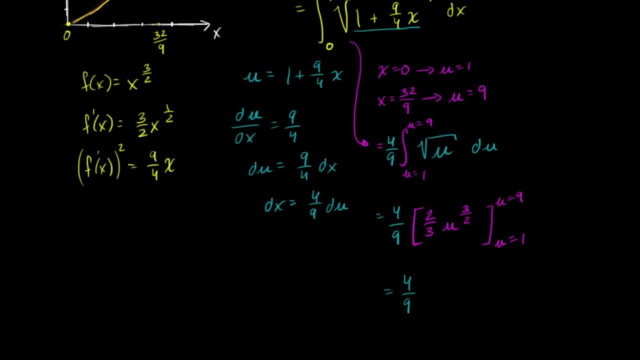 This is going to be equal to four ninths times times, let's see two thirds times nine to the three halves, minus two thirds times one to the three half, so nine to the three halves, that is, let's see. the square root of nine is three. 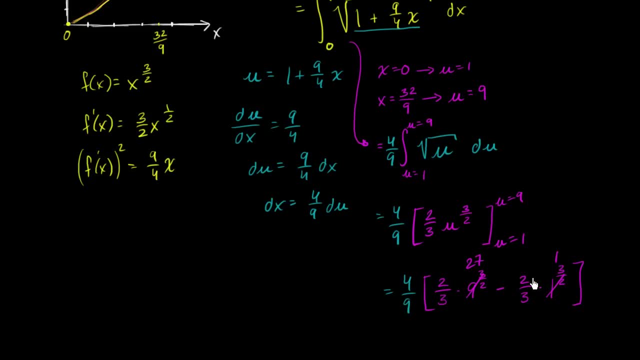 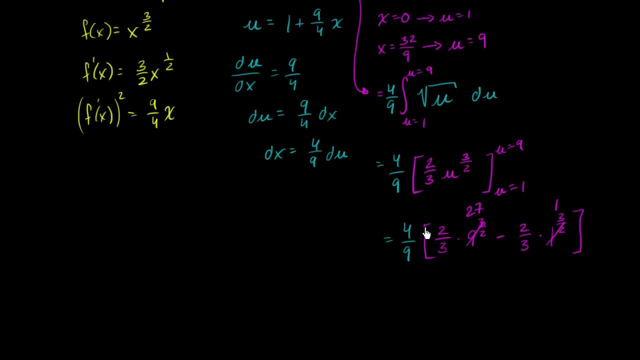 to the third power is 27, and this, of course, is one, so we are left with two thirds of. actually, let's just factor out the two thirds, that makes it easier. so we're going to be left with: